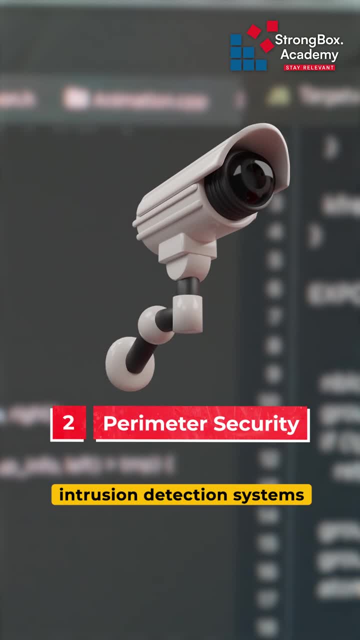 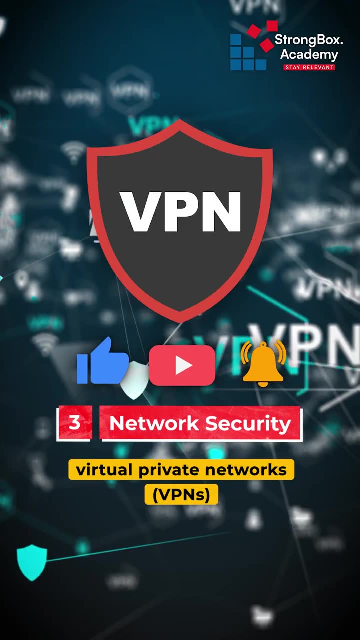 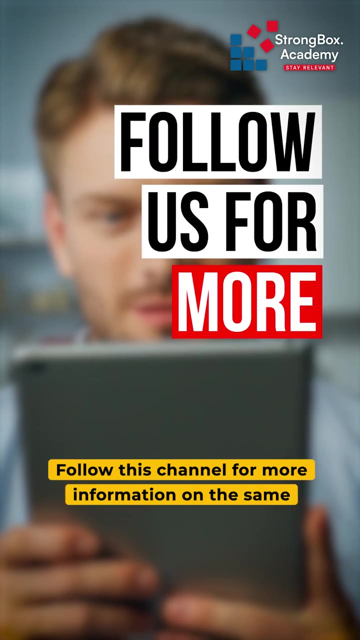 perimeter using firewalls, intrusion detection systems and access control lists. Layer 3 focuses on securing network traffic through encryption, virtual private networks, VPNs and secure protocols. Stay tuned for part 2 video. Follow this channel for more information on the same. 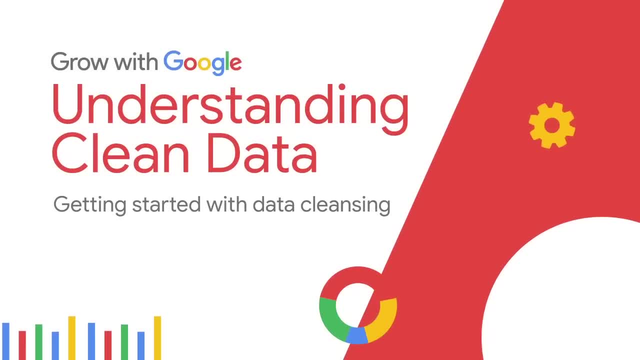 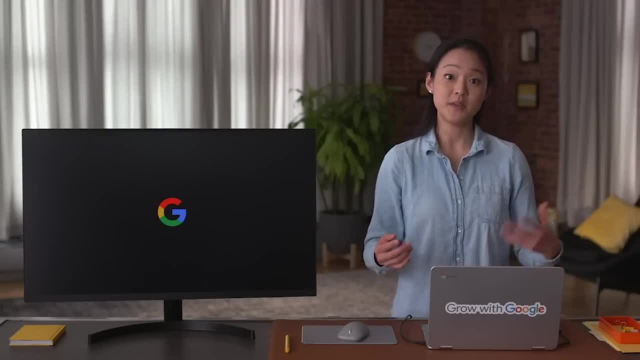 Can you guess what inaccurate or bad data costs businesses every year? Thousands of dollars, Millions, Billions. Well, according to IBM, the yearly cost of poor quality data is 3.1 trillion dollars in the US alone. That's a lot of zeros. Now can you guess? 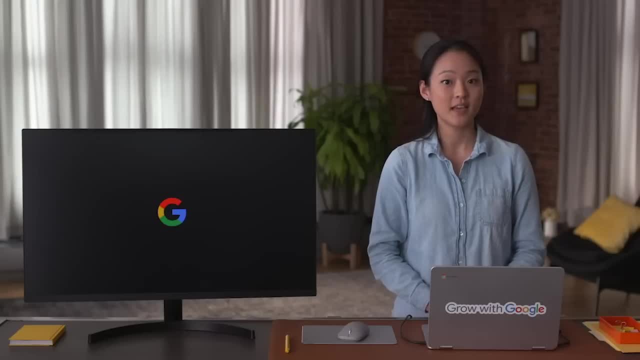 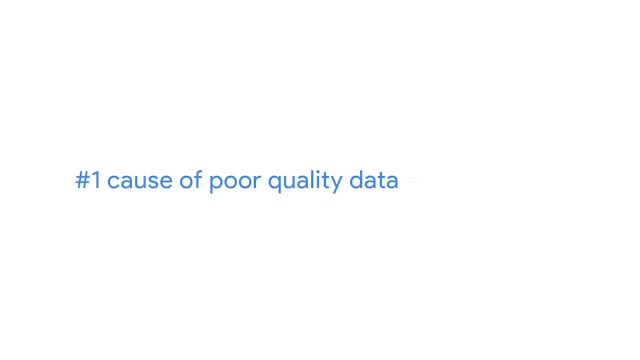 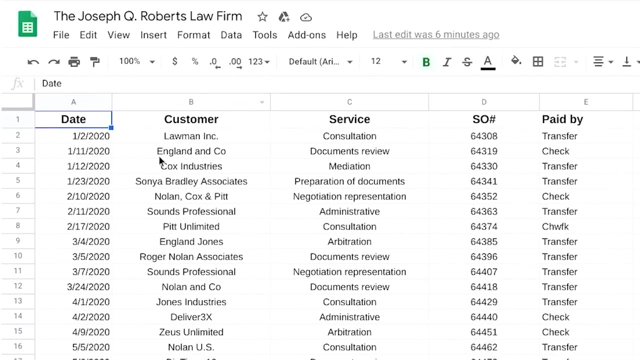 the number one cause of poor quality data. It's not a new system implementation or a computer technical glitch. The most common factor is actually human error. Here's a spreadsheet from a law office. It shows customers the legal services they bought the service. 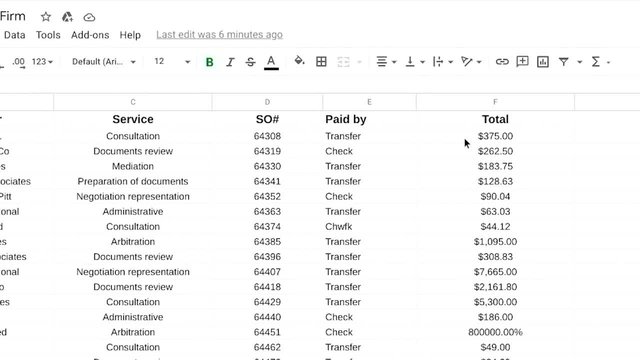 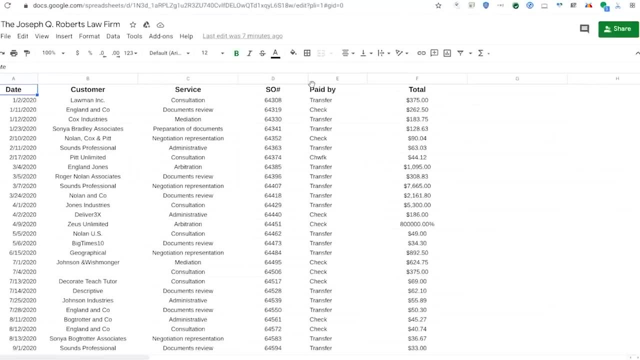 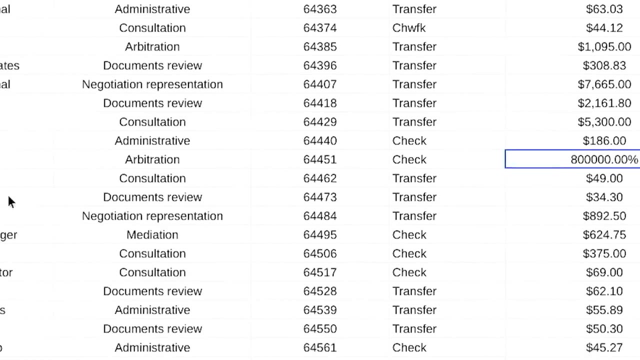 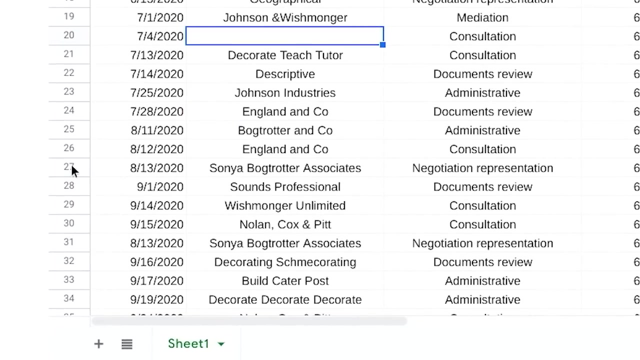 order number, how much they paid and the payment method. Dirty data can be the result of someone typing in the wrong number, Someone typing in a piece of data incorrectly, Inconsistent formatting, Blank fields, Or the same piece of data being entered more than once, which causes duplicates Dirty. 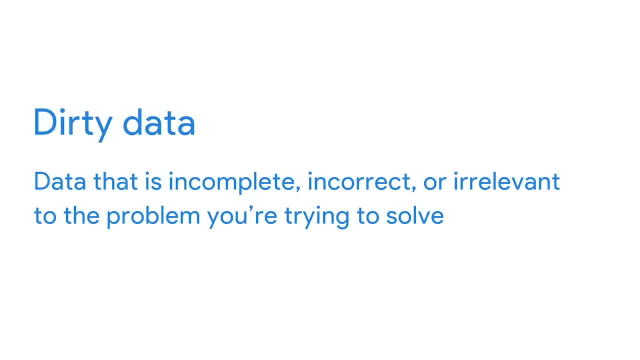 data is data that's incomplete, incorrect or irrelevant to the problem you're trying to solve. When you work with dirty data, you can't be sure that it's incorrect or irrelevant to the problem you're trying to solve. When you work with dirty data, you can't be sure. 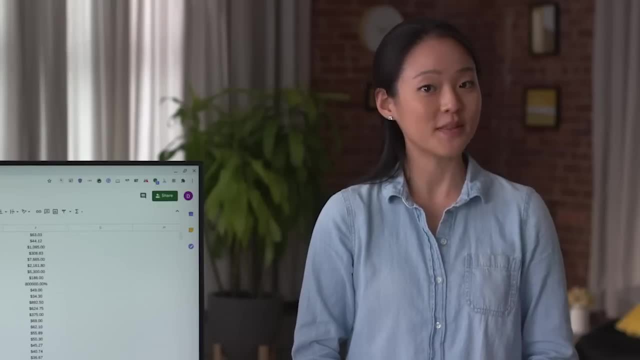 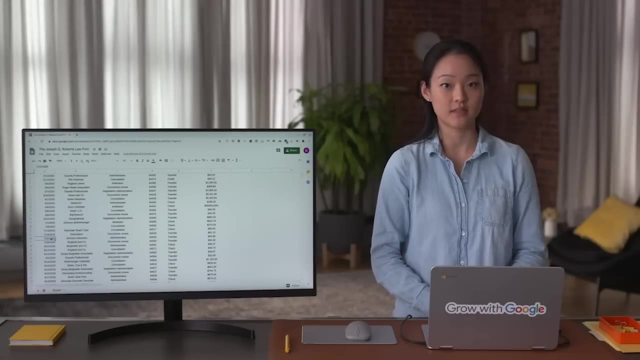 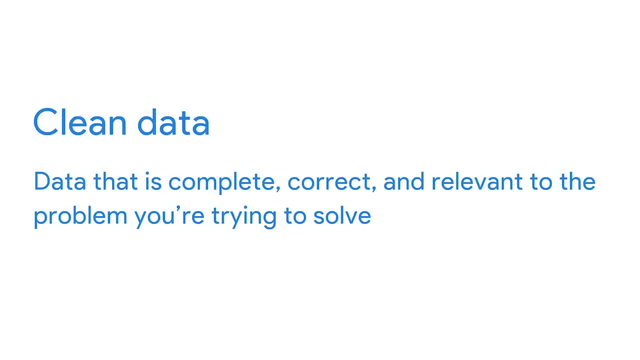 that your results are correct. In fact, you can pretty much bet they won't be. Earlier, you learned that data integrity is critical to reliable data analytics results, And clean data helps you achieve data integrity. Clean data is data that's complete, correct and 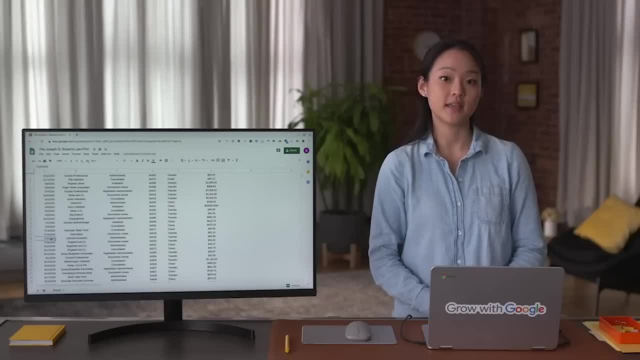 relevant to the problem you're trying to solve. When you work with clean data, you'll find that your projects go much more smoothly. I remember the first time I witnessed firsthand how important clean data really is. I then attempted to scatter the data on the internet to suitable